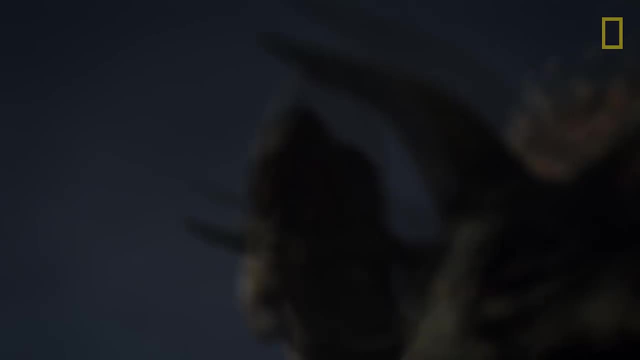 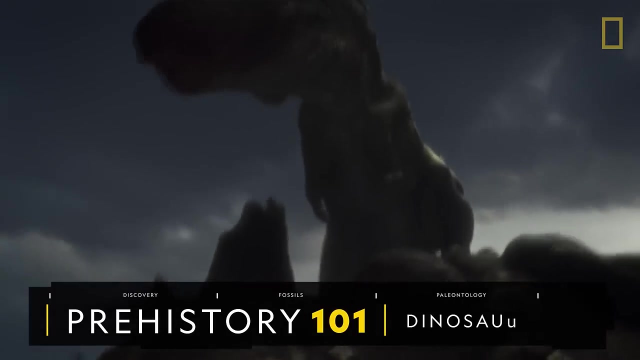 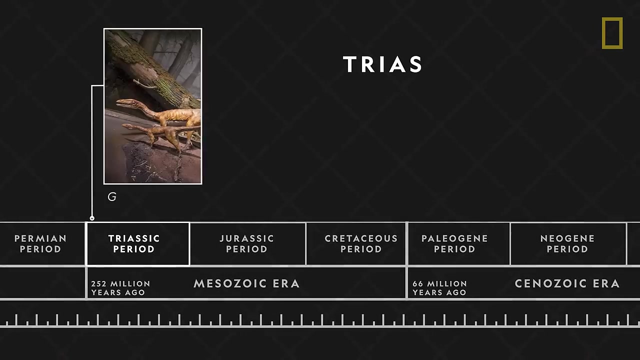 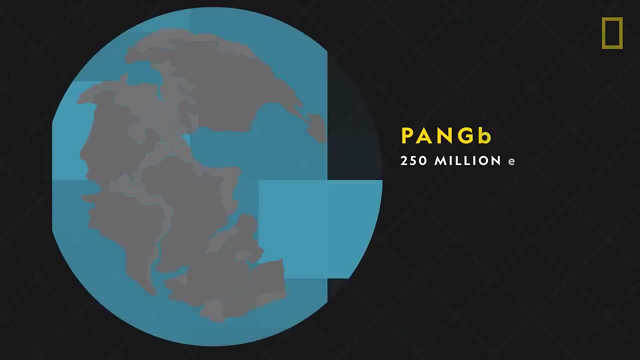 Probably no other creatures on the planet have struck as much fear and awe in our hearts as the dinosaurs. The earliest dinosaurs appeared about 245 million years ago, during the Triassic period, when most of the Earth's landmasses were still joined together as the supercontinent Pangea. 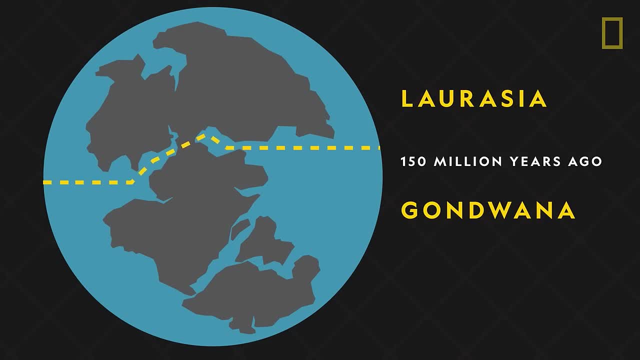 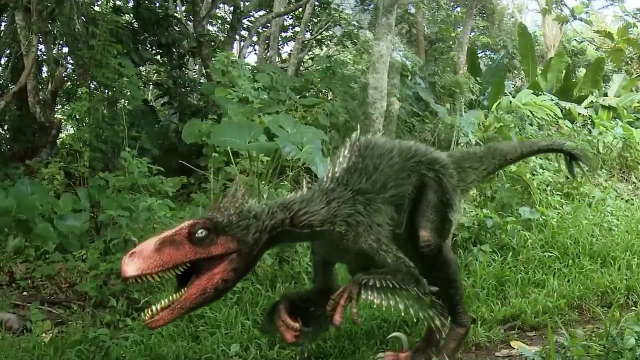 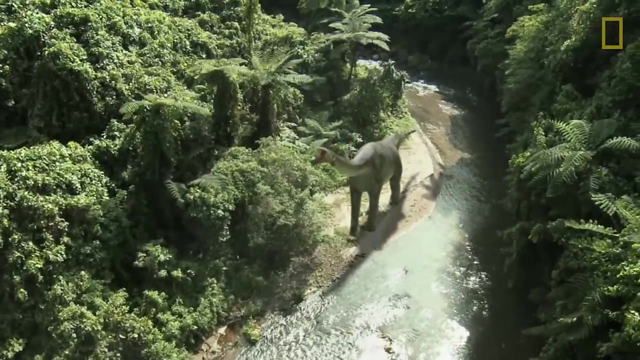 Over millions of years, Pangea split apart, causing the dinosaurs to become separated for the very first time. This led the reptiles to adapt to their specific habitats and diversify, giving rise to many new dinosaur species. According to some estimates, more than 1,000 species of dinosaurs have roamed the Earth. 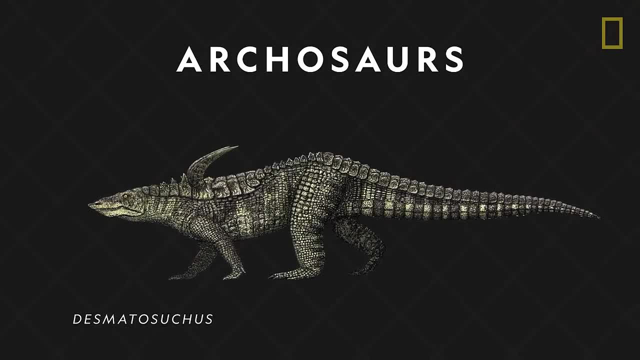 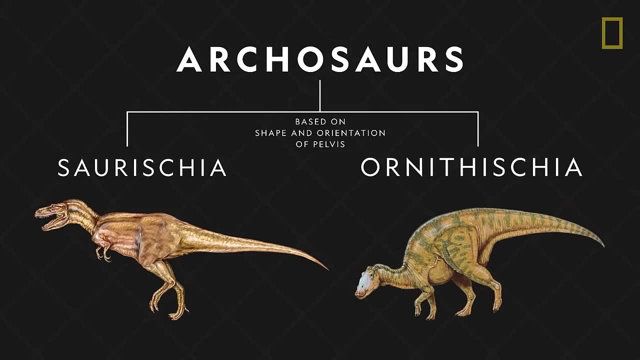 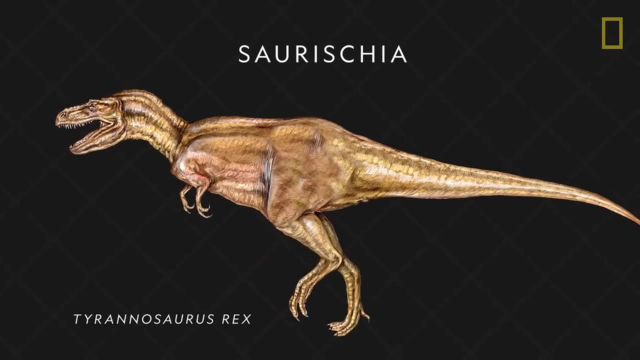 All dinosaurs descended from reptiles called archosaurs. From there, dinosaurs branched out into two major groups, Saurischia and Ornithischia, based on the shape and orientation of their pelvis In Saurischian dinosaurs, such as Tyrannosaurus rex and Brachiosaurus. 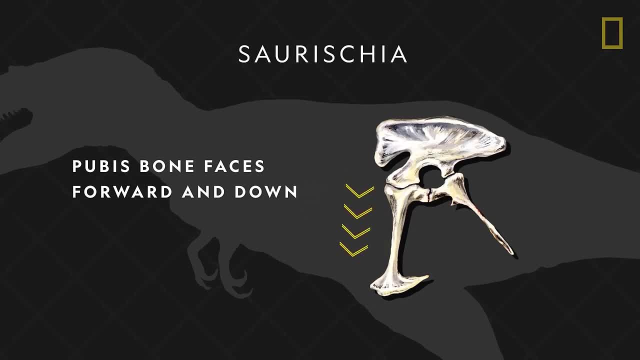 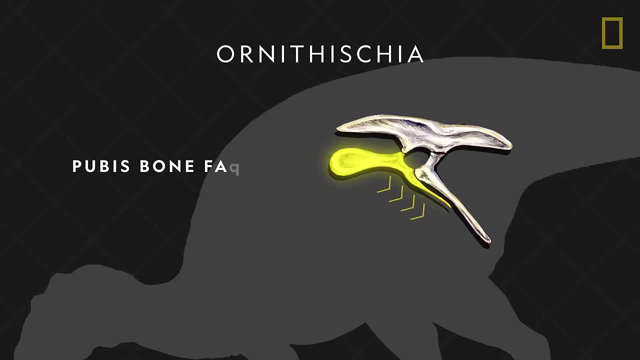 the pelvis's pubis bone faces forward and down In Ornithischian dinosaurs such as Stegosaurus and Hadrosaurus. the pubis bone faces backward and down In Ornithischian dinosaurs such as Stegosaurus and Hadrosaurus. 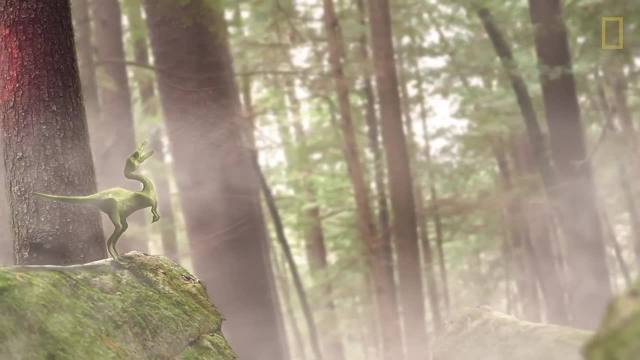 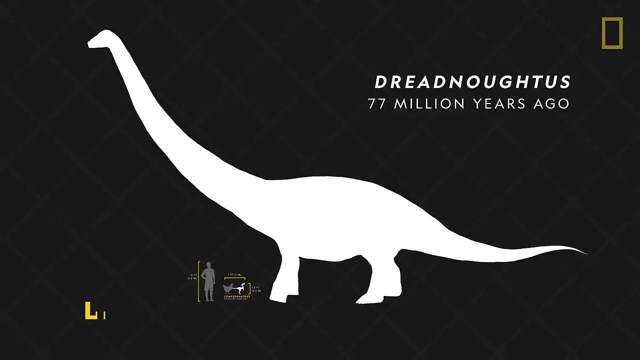 the pubis bone faces forward and down. Across both groups, dinosaurs varied greatly in size. Some were small, like Compsognathus, which was barely larger than a chicken, whereas others were gigantic, like Drednautus, which was 85 feet long and weighed 65 tons. 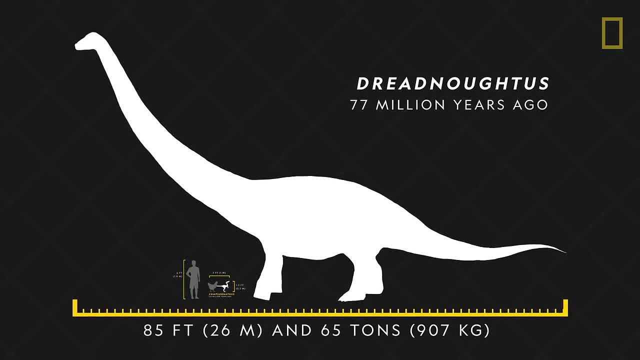 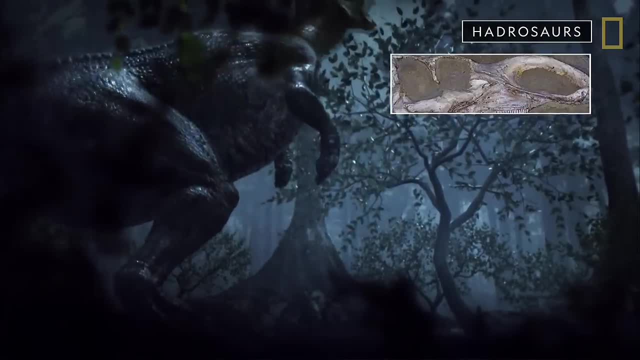 making it the largest land animal to have ever lived. Dinosaur diets varied as well. Herbivores like Hadrosaurs evolved to have specialized teeth. Herbivores like Hadrosaurs evolved to have specialized teeth- teeth for grinding tough plant material. 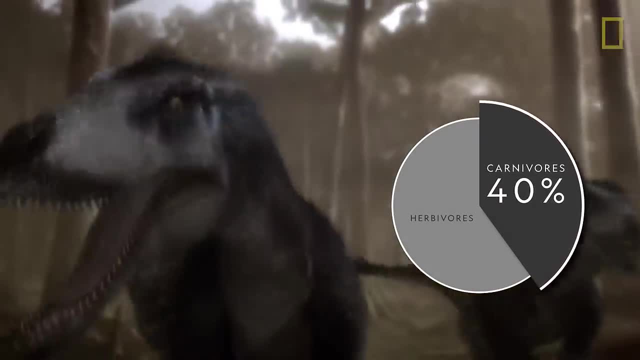 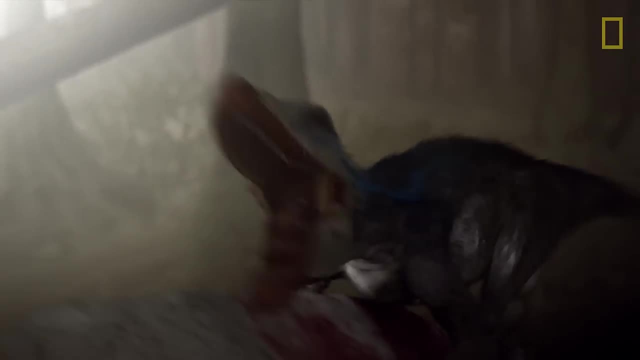 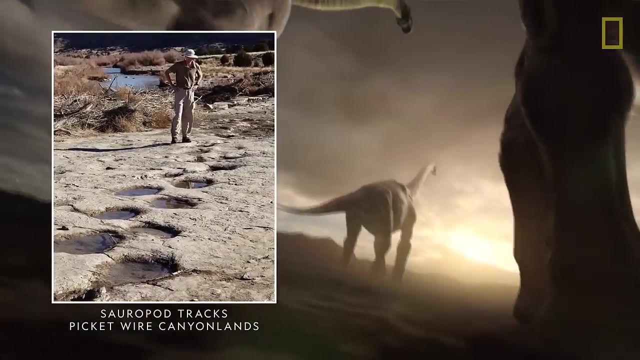 Carnivores made up roughly 40% of dinosaur species. Some predators, like the raptor Deinonychus, even hunted in packs. Social behaviors were also found in other dinosaurs. Footprints and trackways indicate that some of the ancient reptiles traveled together.